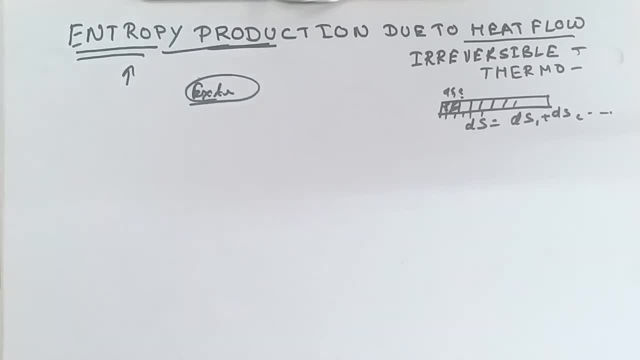 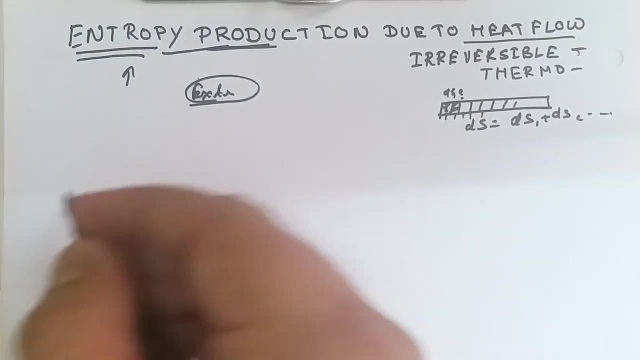 ds2 and so on, so it will be equal to all the entropies. so thus over here, in order to simplify this particular thing, we may split our entropy into two parts. so first is the first entropy, that we may denote it as DES, which is the entropy. 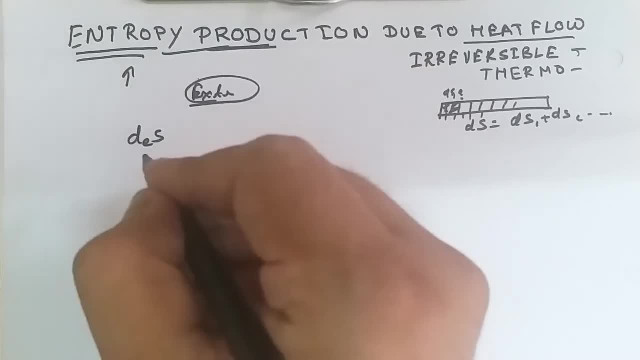 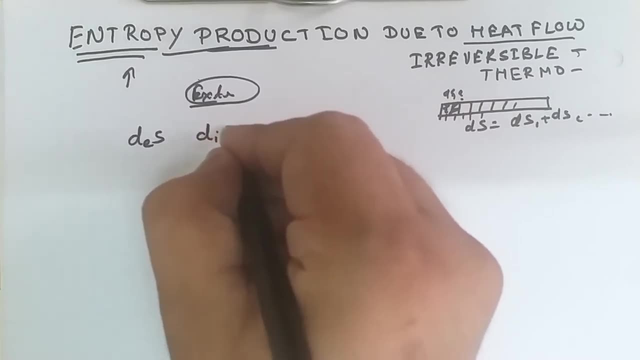 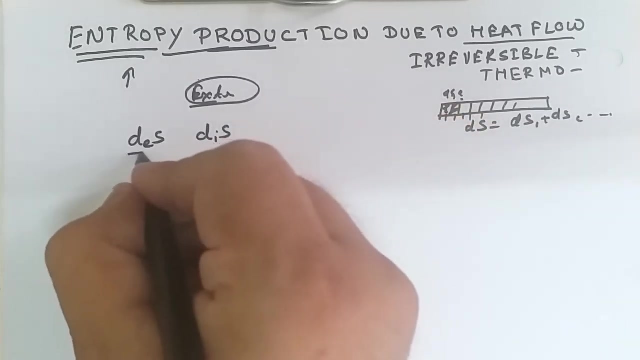 flow due to the interaction with the exterior or due to the interaction with the surrounding. and the second is DIS, which is the entropy contribution due to the change in the inside of the system. so basically, DES is the entropy varying, the entropy change in order to change as we move another system. So we need to figure out the 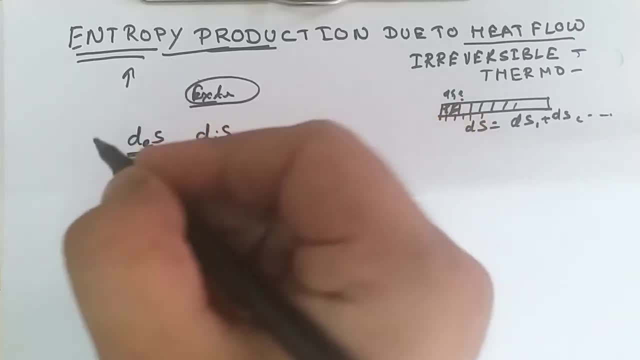 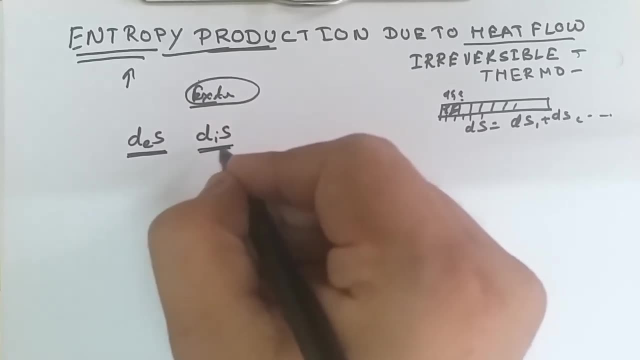 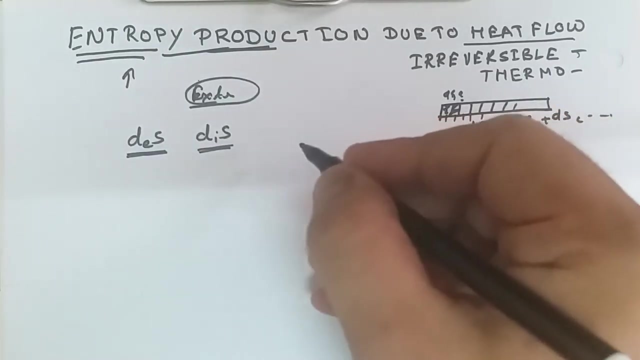 when our system is interacting with the surrounding and that entropy change is referred as DES and DIS is the internal change in the entropy. So let me explain you by taking an example. that is suppose we are performing any particular chemical reaction, say in an RBF. you have in an RBF, you have taken the reactant A and B and you are supplying certain amount of 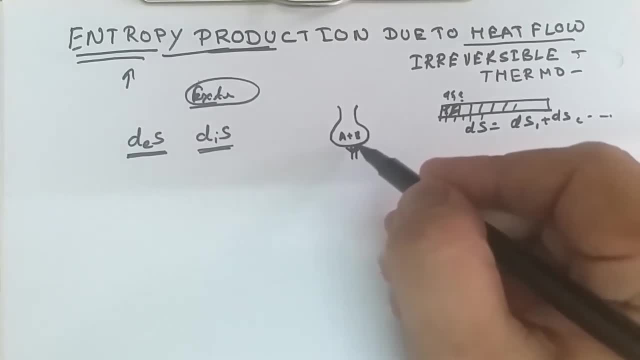 heat. So the flow of heat from the burner or the flow of entropy due to the interaction between the burner and the container or the heat generated, will be our DES. and when the chemicals, that is the entities A and B, they react to give any product, then at that time also there will be 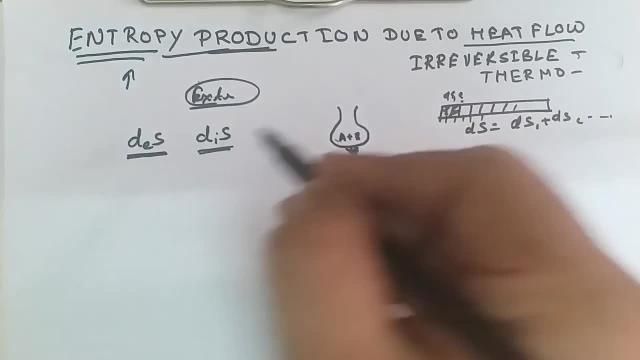 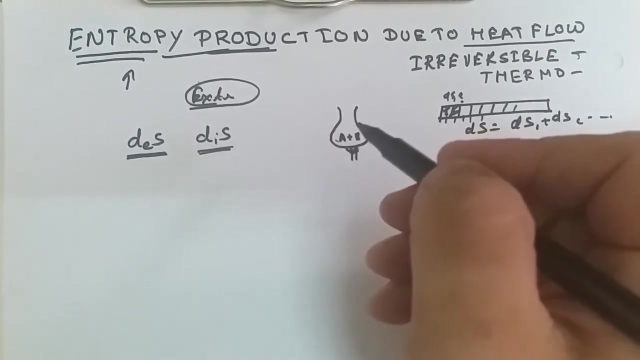 certain amount of entropy change, So that is our DIS. So because of the internal, or when the entropy agentsasse is changing because of the internal contribution, then, or because of the inside of the system, then it will be dis. and when there is an external interaction or when entropy is changing due to the 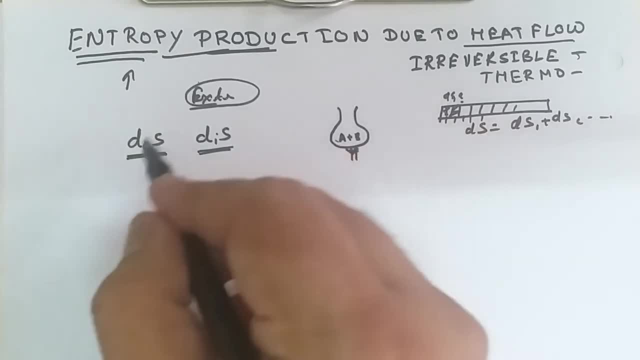 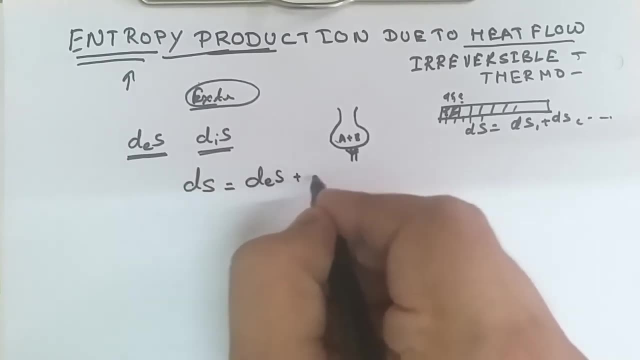 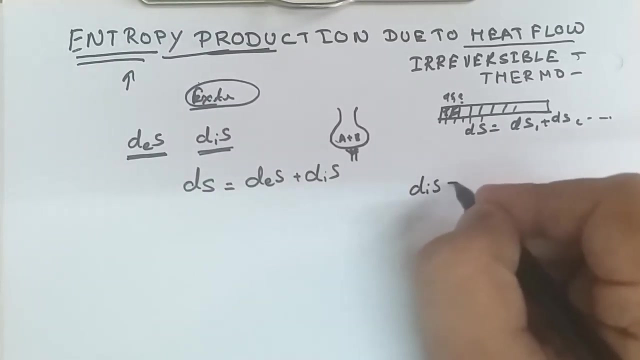 interaction with the exterior of the system or with the surrounding, then it is dis and the total entropy that is ds. we may write it as des plus d i s. okay, and over here, dis is equal to zero for a reversible, for a reversible process, for a reversible process, and always dis is greater. 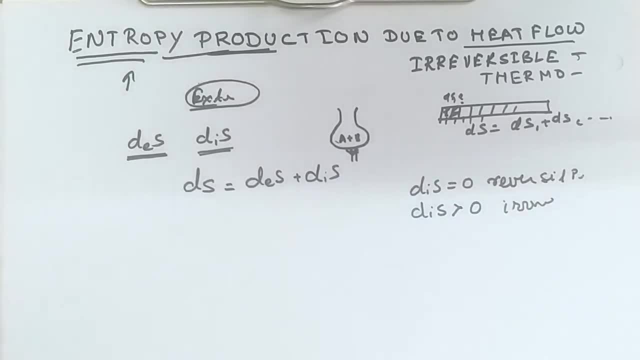 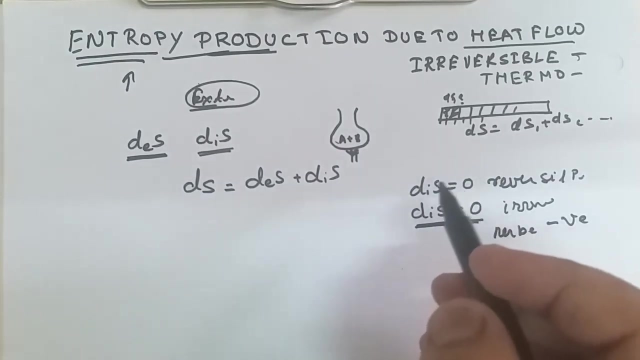 than zero for an irreversible process. so always, always when d is, d is should be greater than zero, greater than zero for an irreversible process that we are looking at and further. this quantity can never be a negative one. so d is can never be negative one, and this d is is our entropy. 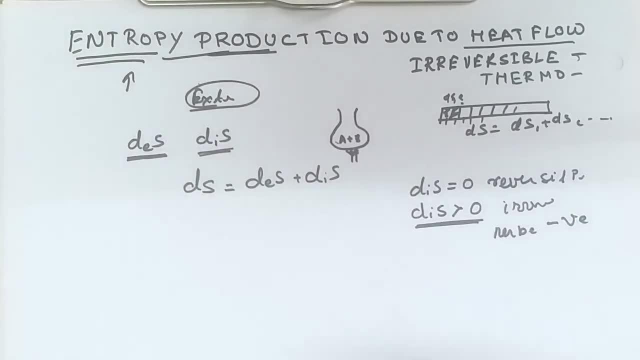 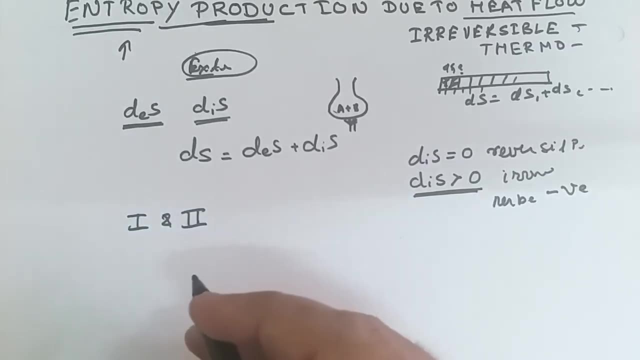 production, because this is the entropy which is produced. now suppose if we consider that our system is made up of two phases, that is, phase one and two, which is the entropy of this system maintained at two different temperatures. that is, phase 1 is maintained at temperature T1. 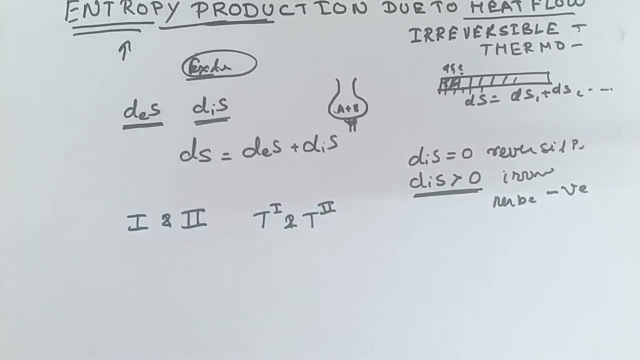 and phase 2 is maintained at temperature T2 and we have already studied the second law of thermodynamics which says that ds is equal to. we have dq upon T, where dq is the heat received from the surrounding and T is the temperature of the system and always as told, ds will be. 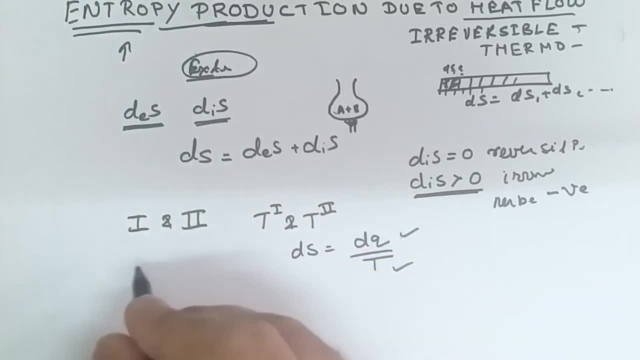 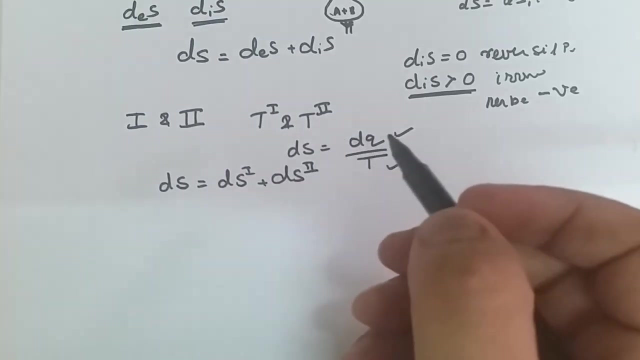 positive now for this particular system, when our system is divided into two phase. okay, as you have earlier also seen that when our system is divided into small number of phases, then the total entropy, ds, will be equal to ds1 plus ds2 and as entropy is splitted, also the heat received, that is dq. 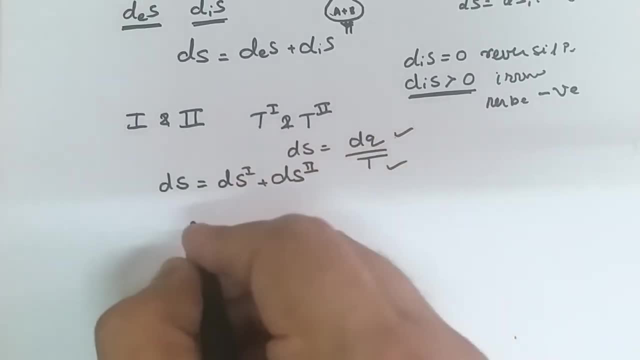 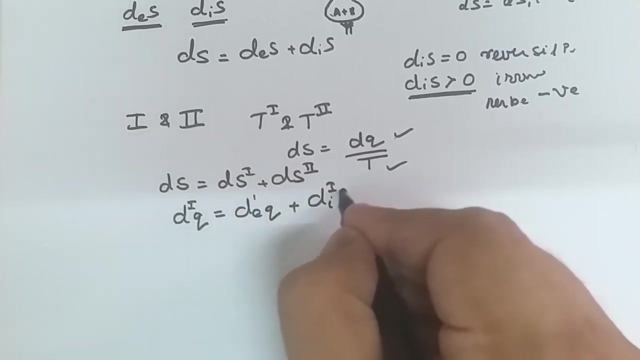 will also be splitted into the two quantities. that is heat, heat received, that is, we can write this as d1 cube, that i can write this d1 e cube plus d i 1 cube. so this is our heat because of the external interaction and this is. 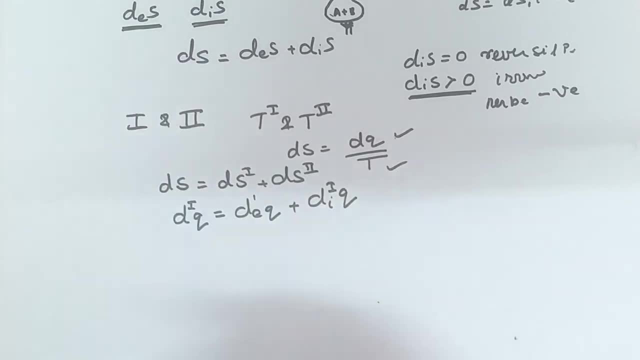 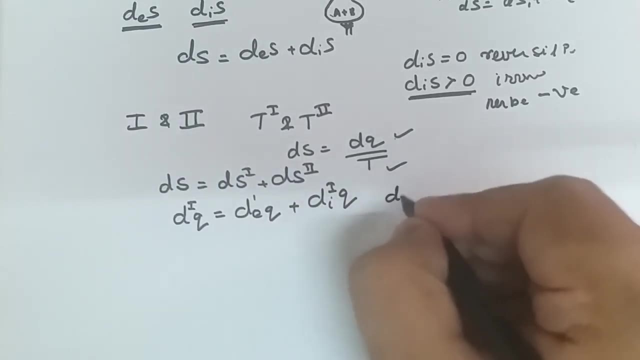 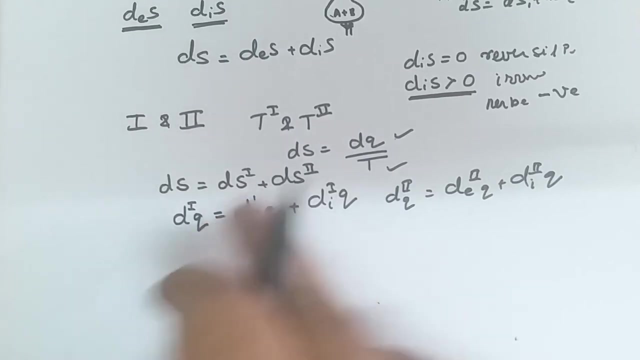 the internal generation, because the reaction may be exothermic or an endothermic reaction, so there may be the heat change. so similarly for the second system, that is d2 cube, we can write it as d e2 cube plus d2 i cube. okay, further we may substitute this terms in this particular. 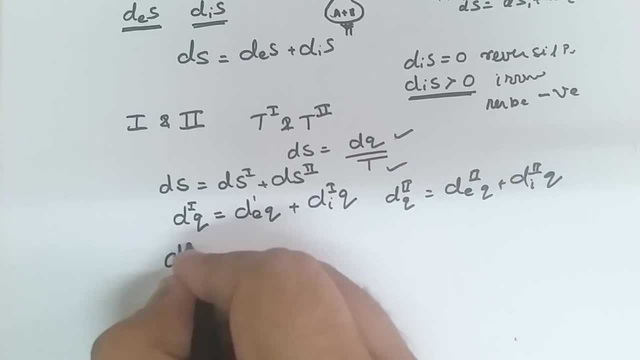 expression that means we can write. we can write: d1 s is equal to d1 cube upon d2, i cube, sorry, t1, and that we can write it as d e i cube upon t1 plus d i 1 cube upon t1 and similarly. 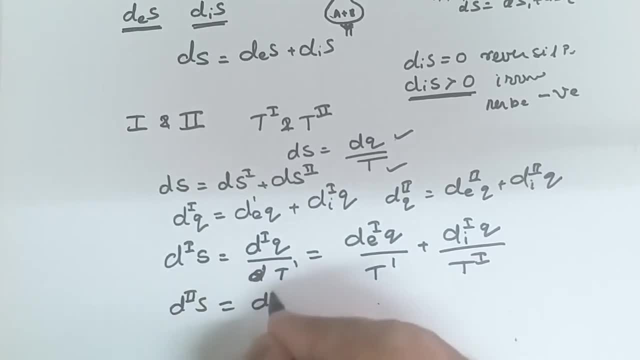 for the second case, that is, that will be d2 cube upon t2, that is equal to d e 2 cube upon t2 plus d e 2 cube upon t2. okay, so these are the two cases and when we combine this, that is, we have written that our 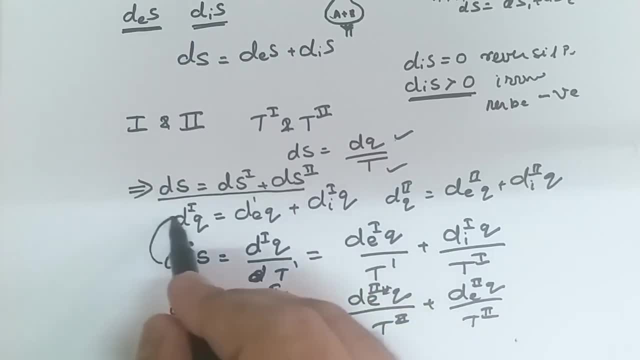 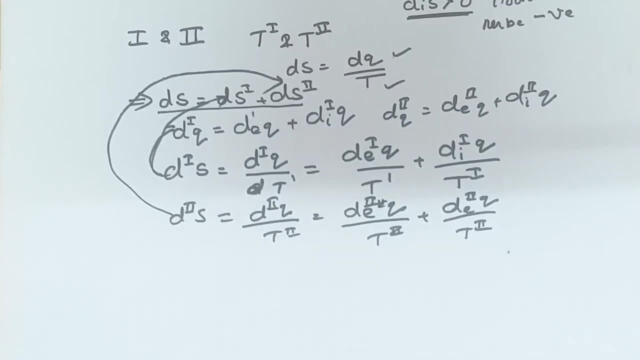 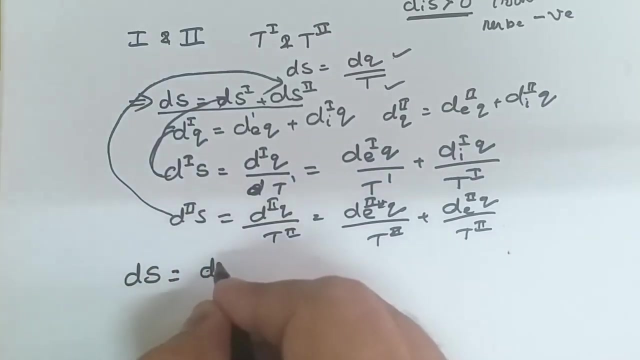 total entropy ds is equal to this, so values of this can be substituted over here and this also can be substituted over here, and hence our expression, and will be equal to. we can write ds that is equal to d 1 e q upon t 1 plus d 2 e q upon t 2 plus d i t i 1 q into 1 upon t i minus. 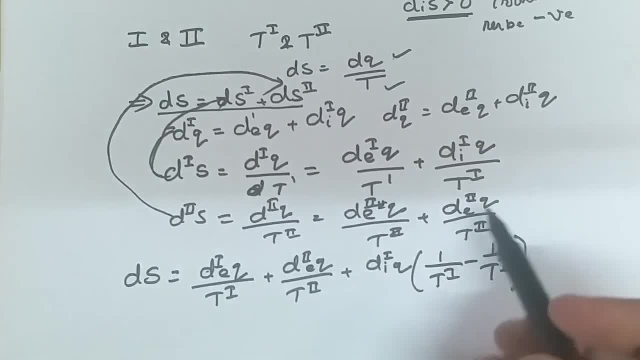 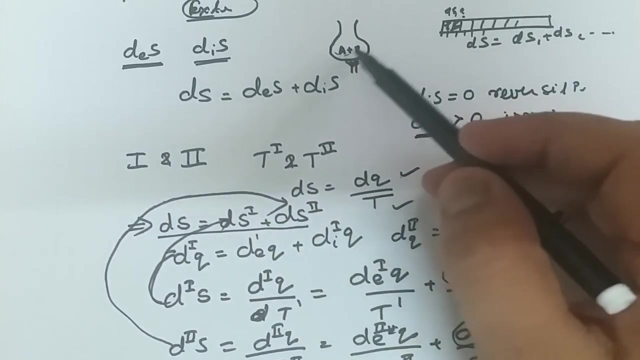 1 upon t 2. okay, so over here from both. this we can take because the heat, the internal heat for the system will be same. that is, uh, as we have taken two components over here, also suppose we can consider two components, a and b, so the internal heat for both the components will be. 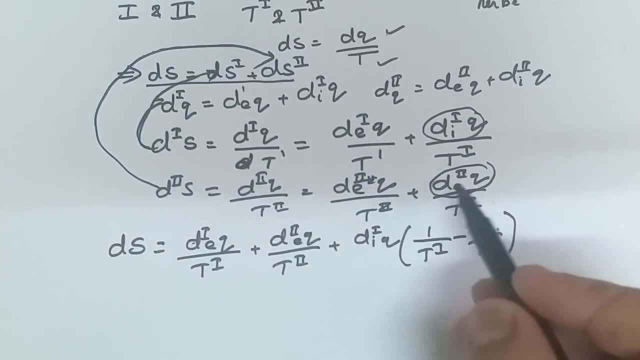 same. so over here: in place of b, q and d 2 e- sorry, d 2 i q- i will substitute only d 1, and hence everything remains same. okay, now over here. in this expression, the first two terms it represents our des and this term it represents dis, which is our entropy production. 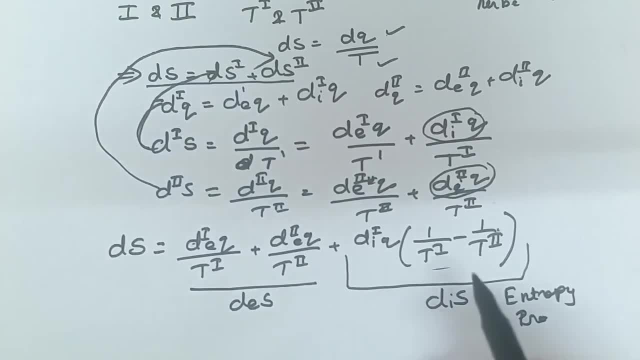 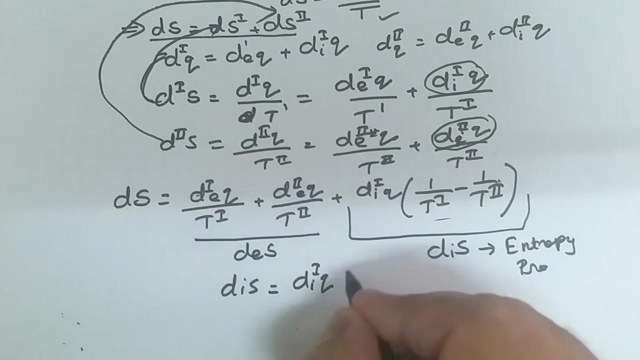 arising due to the transfer of heat from phase 1 to phase 2. okay, and this is our, and this transfer of heat basically arises from phase 1 to phase 2 as because of the temperature difference. okay, and hence this we can write it as: d is that is equal to d. i 1 cube into 1 upon. 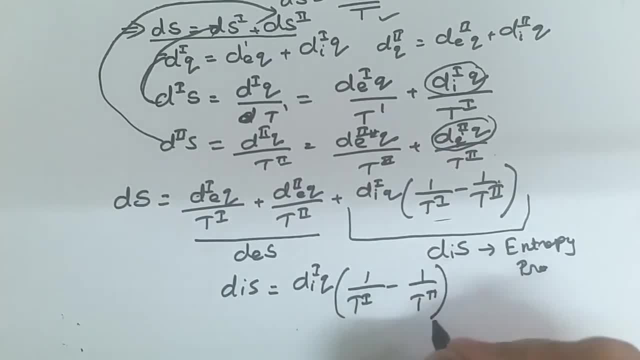 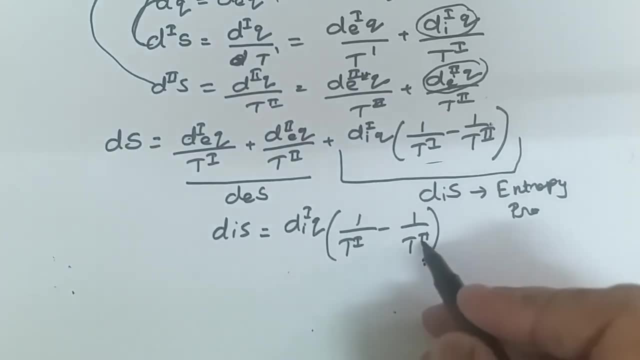 t i minus 1 upon t 2, and over here in this expression we can see that if t 2 is greater than t 1, then and then d i s will be greater than 0, and in that case d i s will be greater. 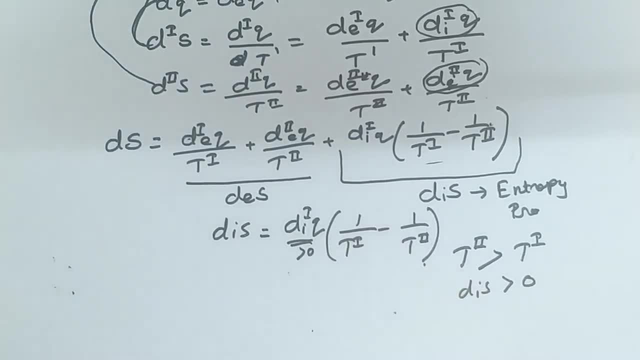 than 0, since this quantity is always greater than 0. okay, and even if we have t 1- sorry, t 1 is greater than t 2- then under such circumstances also, d i s will be greater than 0, because under such circumstances the value of d i cube will be less. 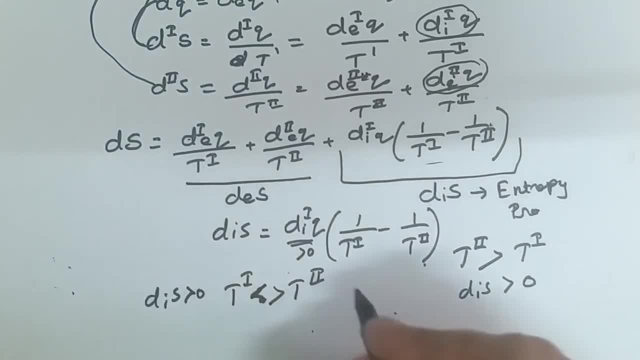 than 0 and, as a result, the whole system or the our value of d i s will always be greater than 0, as we have seen you earlier. further, the value of d i s will only be equal to 0 when our system is under thermal. 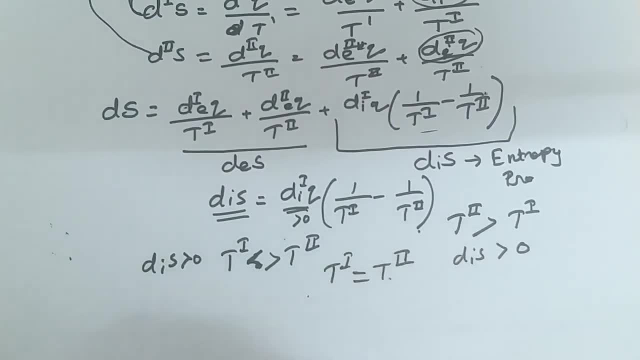 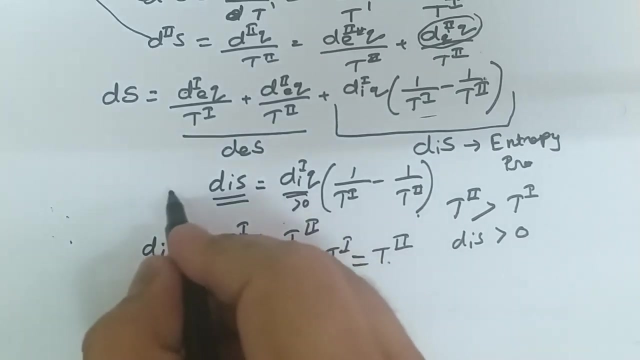 equilibrium, that is, when t 1 is equal to t 2. at that time d i s will be equal to 0 and under such circumstances, our system will be a reversible system, and that we are not very much interested. okay, so hence this expression. that is, this expression can be written in the form that is sigma. 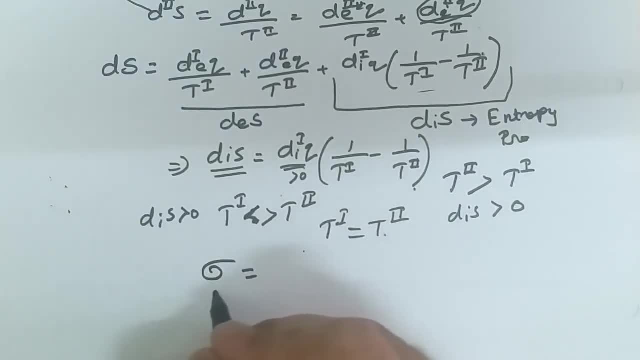 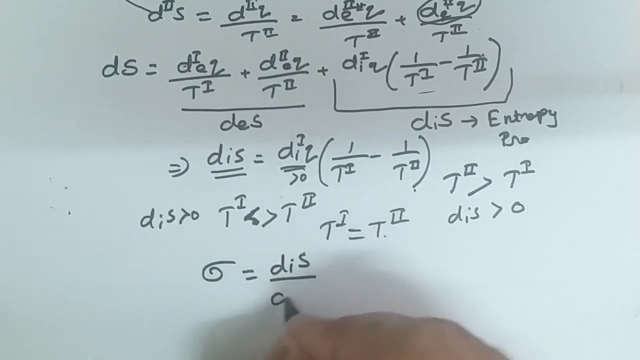 so we are representing the entropy production in the form of sigma and hence we are writing: sigma is equal to. we may write it as generally the entropy production is written in the form of entropy production per unit time and hence the entropy production per unit time, we may write this: